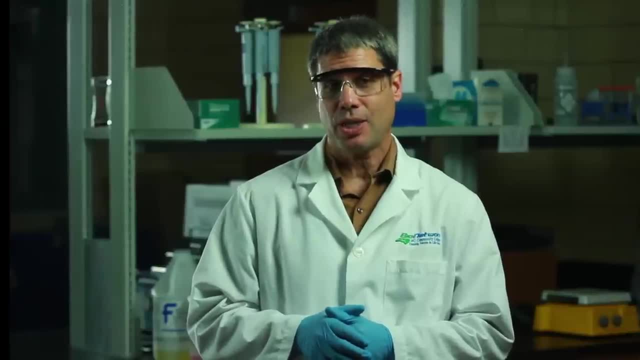 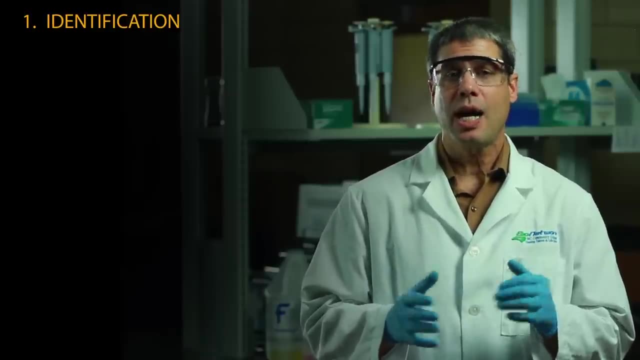 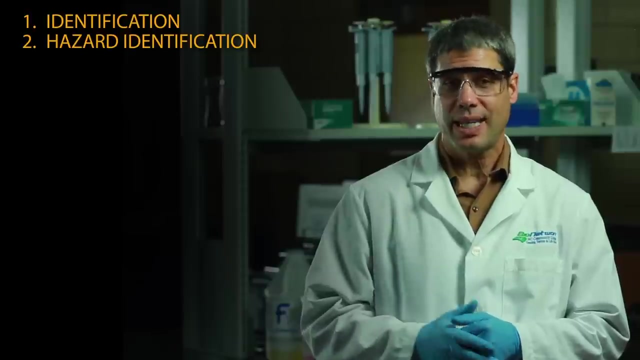 SDS must now be organized into 16 sections. Section 1, Identification: Here you'll find the chemical's name description and the manufacturer's contact information. 2, Hazard Identification: This section lists signal words, warnings and safety symbols. 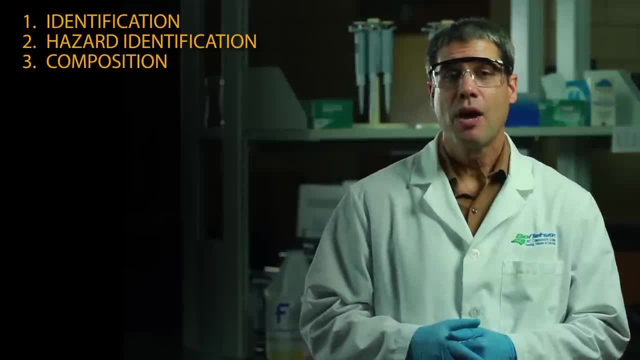 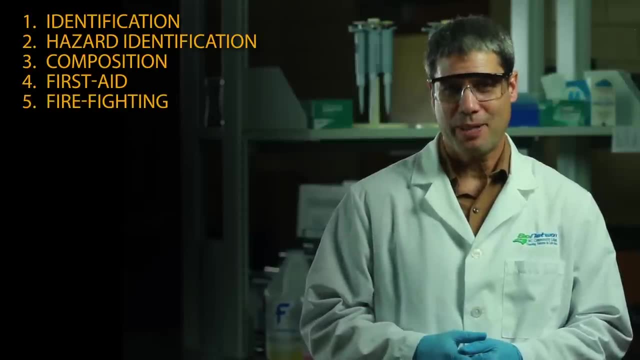 3, Composition- A list of ingredients. 4, First Aid Measurement. 3, Composition- A list of ingredients. 4, Firefighting Measures. What's the required treatment for a person who's been exposed? 5, Firefighting Measures. 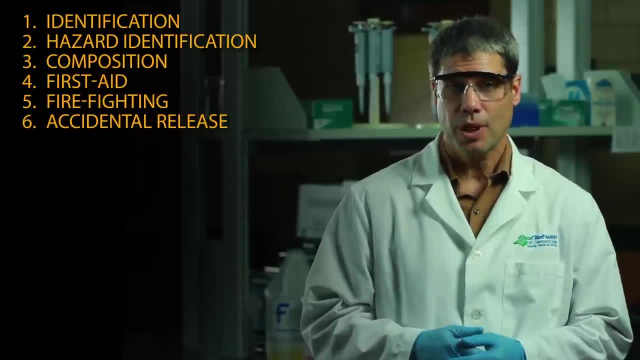 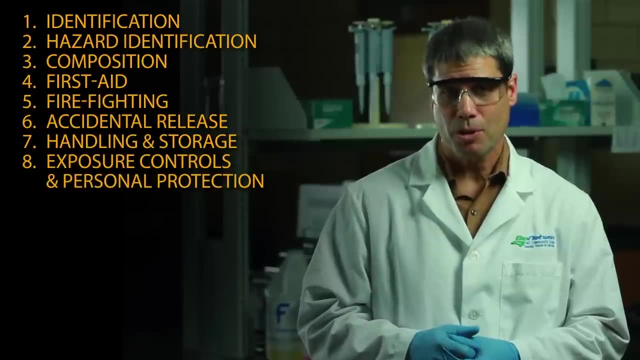 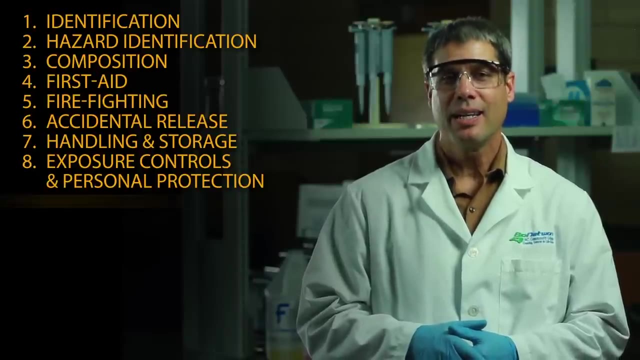 6, Accidental Release Measures. These are instructions for containment and clean-up of spills or leaks. 7, Handling and Storage Requirements. 8, Exposure Controls and Personal Protection. This describes OSHA's exposure limits and recommendations for PPE. 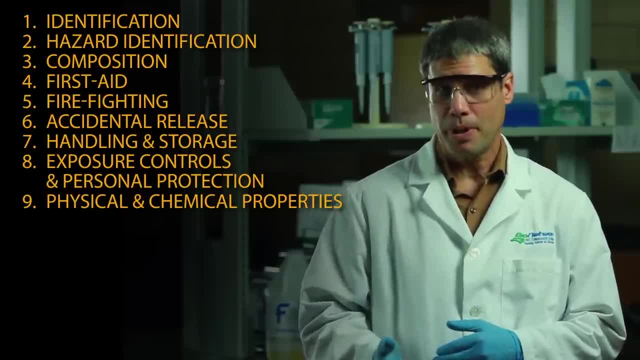 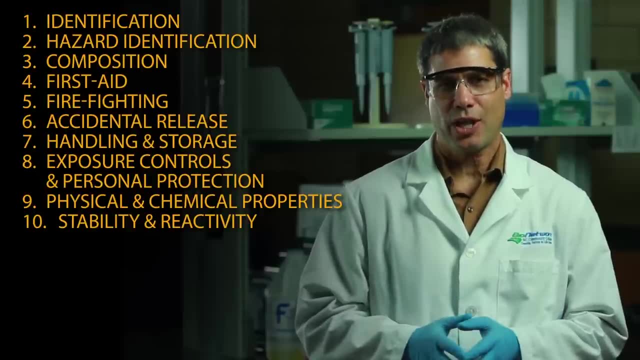 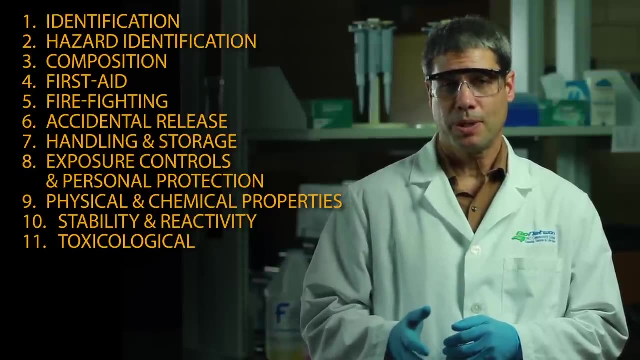 such as appearance, odor, pH, flashpoint, solubility and evaporation rate. 10. Stability and reactivity: How to avoid hazardous reactions. 11. Toxicological information: Find out about the likely roots of exposure symptoms, as well as short and long-term effects. 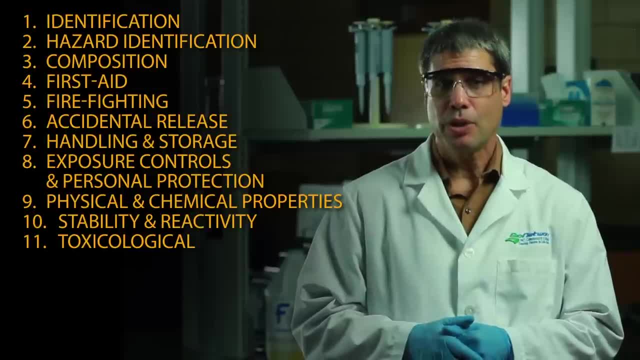 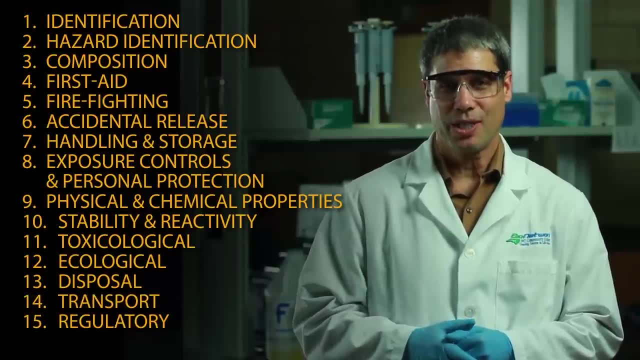 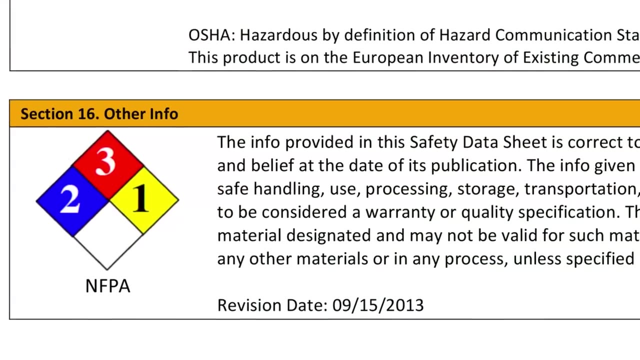 Sections 12 through 16 aren't mandatory, but you should at least be familiar with them. 12. Ecological Disposal, Transport and Regulatory Considerations. Section 16 is for any other pertinent information. This is where you'll find the date that the SDS was prepared, along with the last known revision. 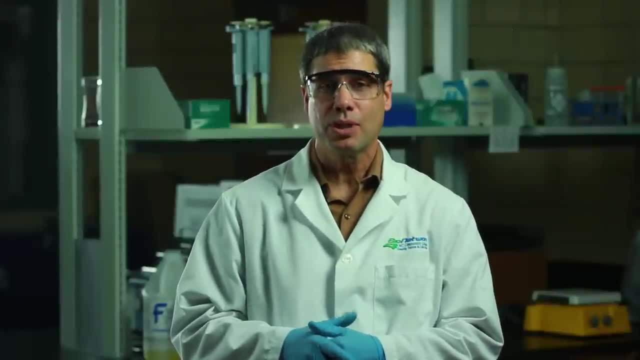 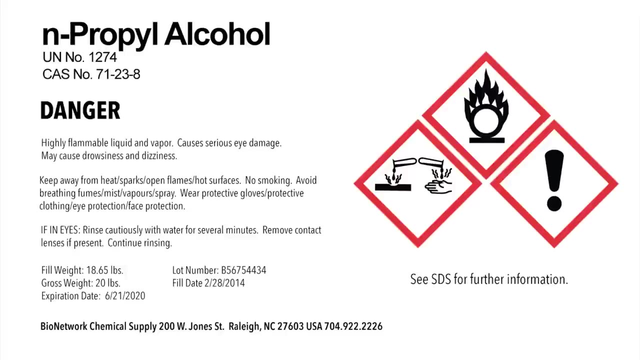 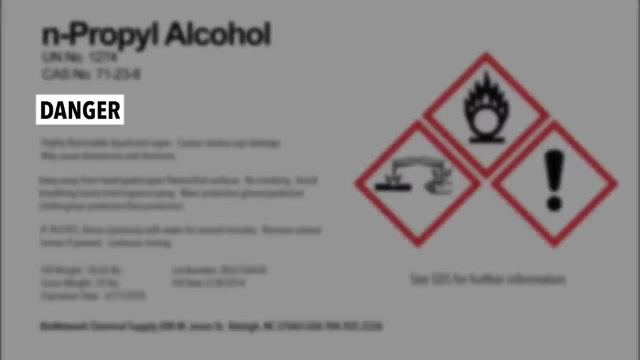 Safety data sheets provide a lot of information about how to use chemicals safely in the lab, But there's also another way to learn about a chemical, and that's by reading its label. The new GHS format requires each chemical inlibrary. The label is then labeled with the product name, a signal word, such as danger or caution. 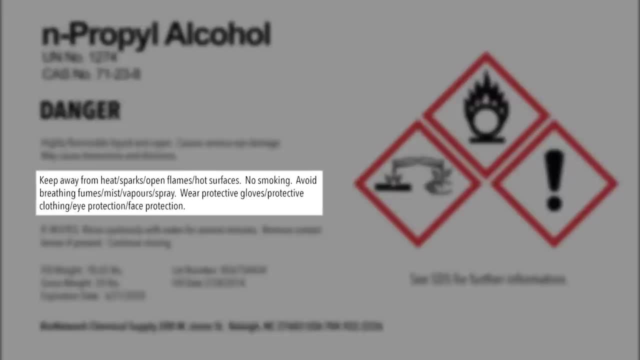 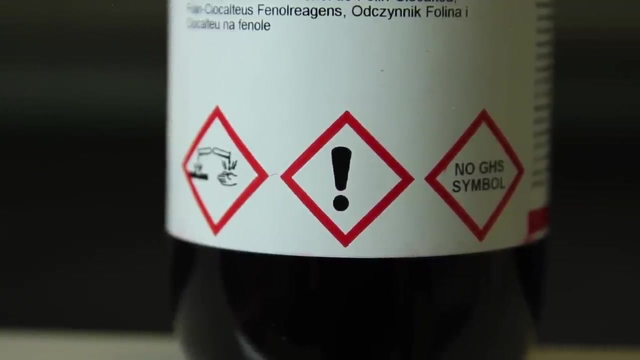 physical health and environmental hazard statements, precautionary statements, pictograms, first aid instructions and the supplier's contact information. Pictograms consist of a symbol on a white background framed in a red border. Each pictogram represents a specific hazard. 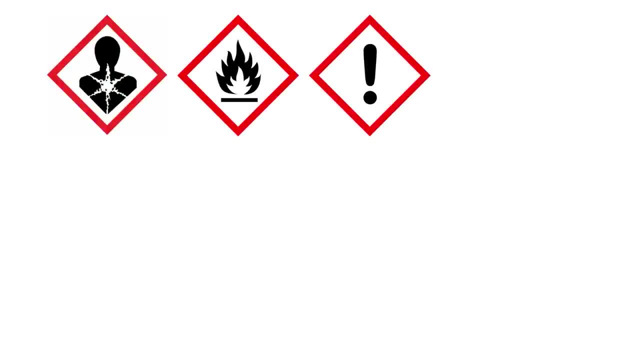 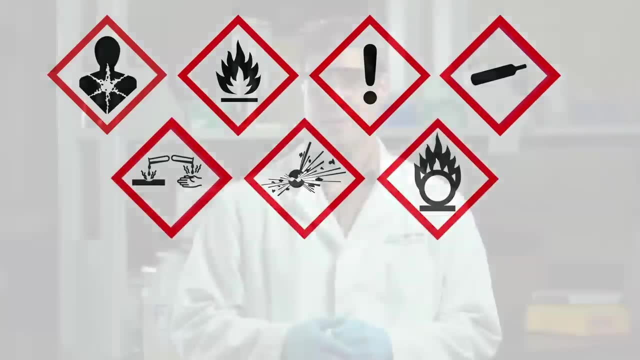 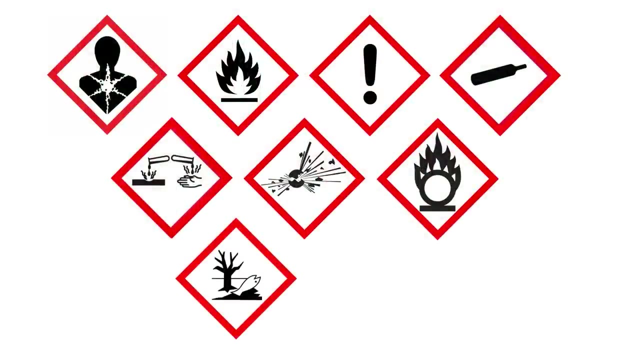 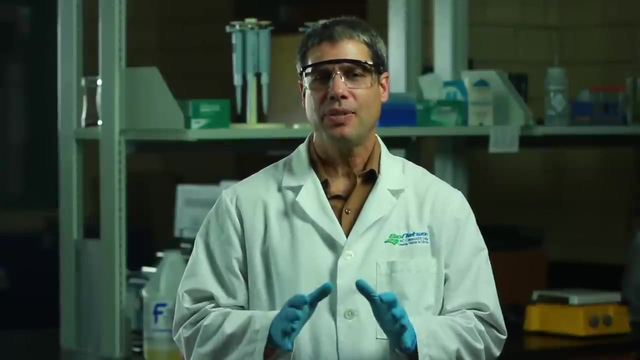 Health, Flammability, Toxicity, Compressed gases, Skin and eye protection, Unstable explosives. Oxidizers: An oxidizer is a chemical that initiates combustion through the release of oxygen, Environmental hazards And acute toxicity. Now you know how to identify potential chemical hazards by looking at both safety data sheets and chemical labels.